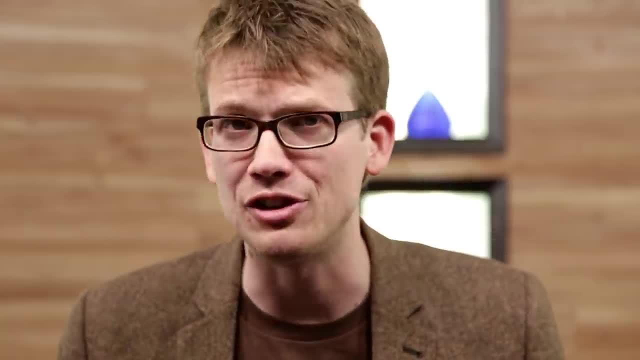 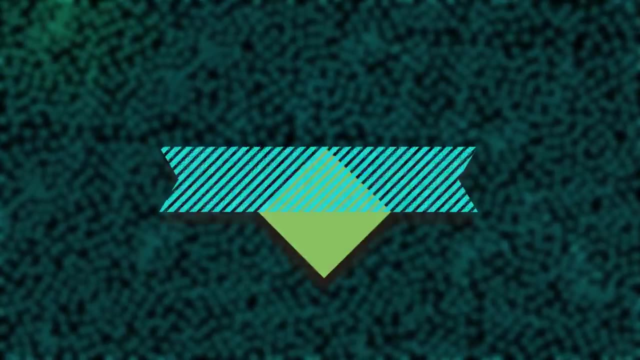 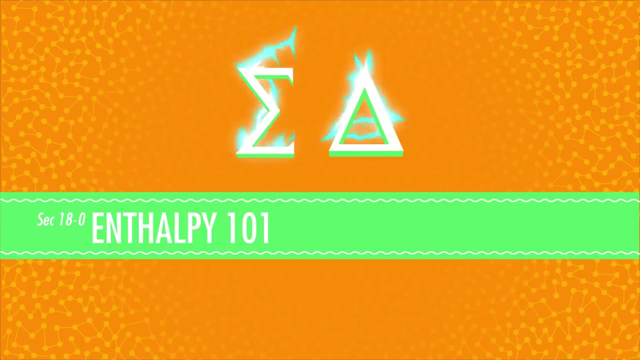 How much energy? Well, that is not the simplest question to answer, And yet today we shall answer it, Kinda Using a nifty little thing called enthalpy. Last time we learned about internal energy and the two ways that it can be transferred. 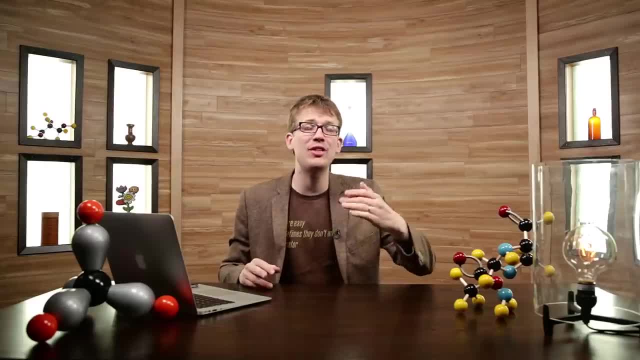 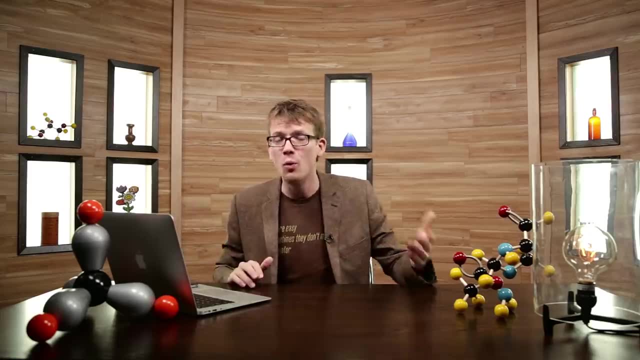 By heat or by work. And heat and work are useful concepts but they have limitations, Particularly that it is extremely difficult to figure out how much of which one is being done. Work is energy transferred to the motion of objects, While heat is energy transferred to the motion of atoms and molecules. 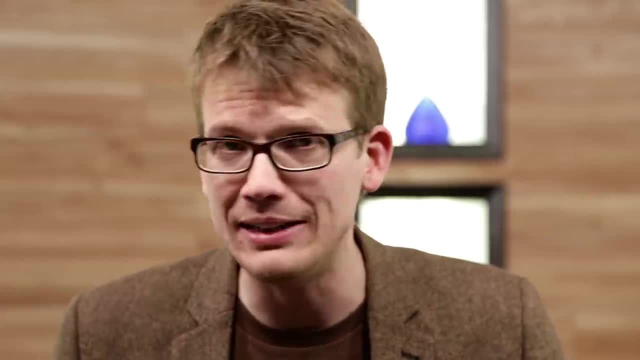 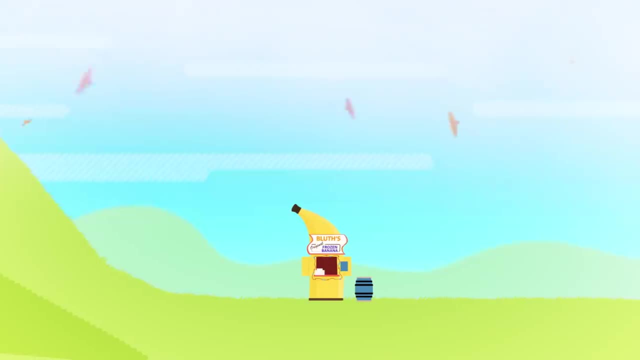 But for any given change in energy, the split between work and heat could be pretty much anything, As long as there's some going to each Say: my car is at the top of a hill and there's a frozen banana stand at the bottom. 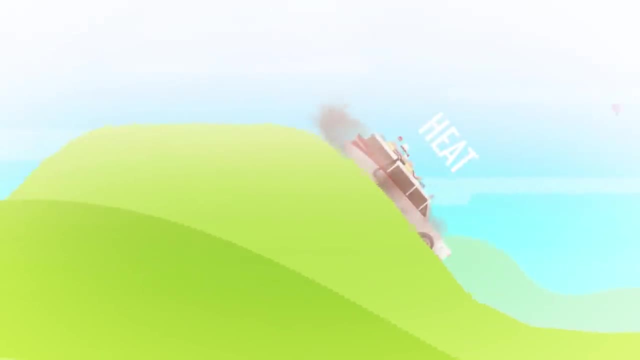 If I roll down with my brakes on, lots of heat will be transferred into my brake pads and my brake discs And I will kind of like very slightly knock into the frozen banana, Doing a tiny amount of work on it. But if I am reckless and insane, very little heat will be generated. 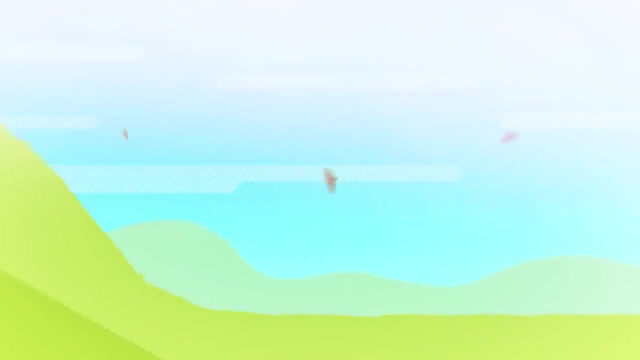 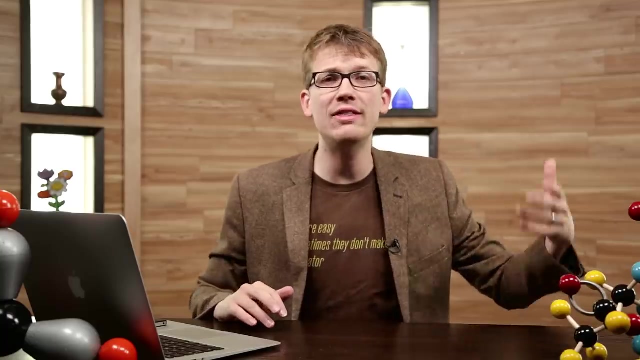 And my car will do a huge amount of work on the frozen banana stand. Both paths transfer the same amount of energy, But one produces very little heat and the other produces a ton. And so we say that heat and work are pathway dependent. The amount of heat or work done depends on the pathway you take. 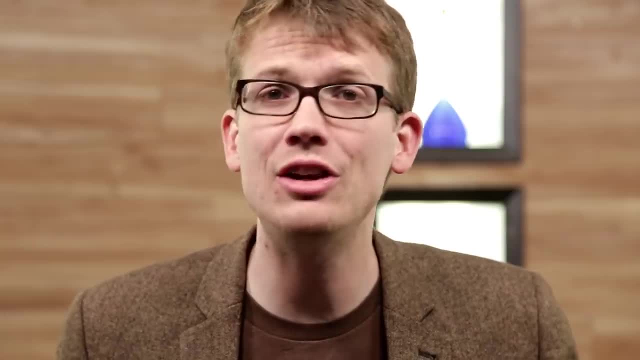 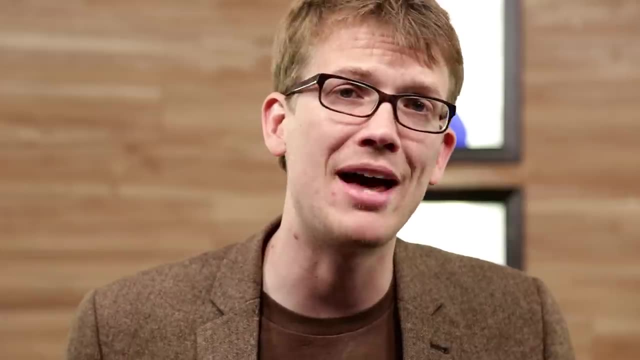 The change in energy, on the other hand, is the same in either case. Change in energy is independent of the pathway. In chemistry, in physics, in math, we call that a state function, Because the only thing that matters is the starting state and the ending state. 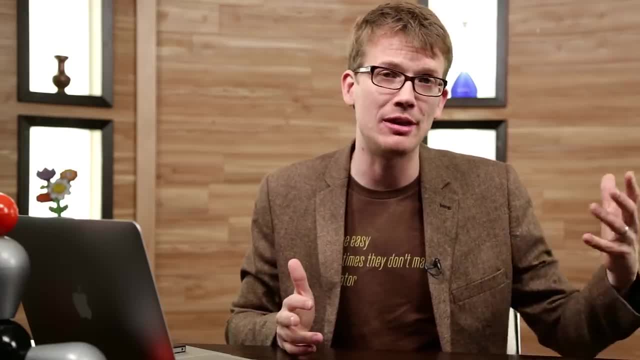 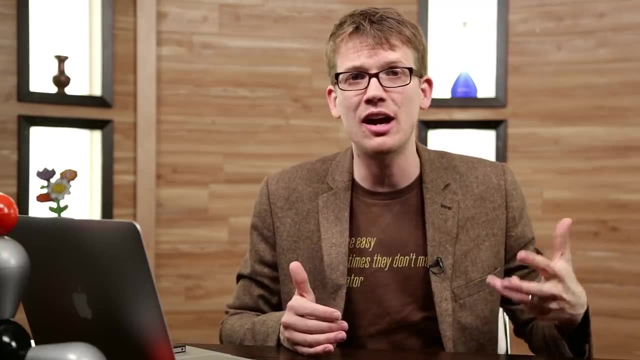 Not the stuff in between, Not how you got there. State functions are pretty great because they make the math very simple. It's just one amount minus another amount. It would be pretty fascinating to know exactly how much energy is tied up in a molecule. 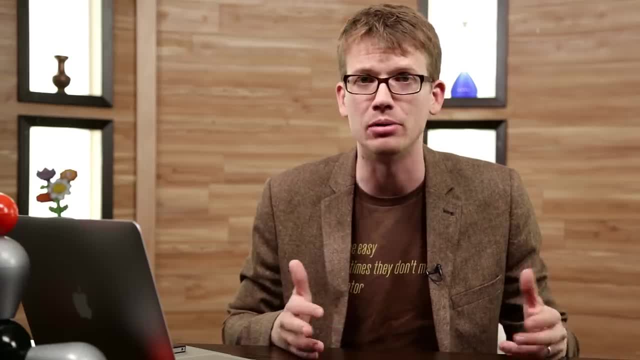 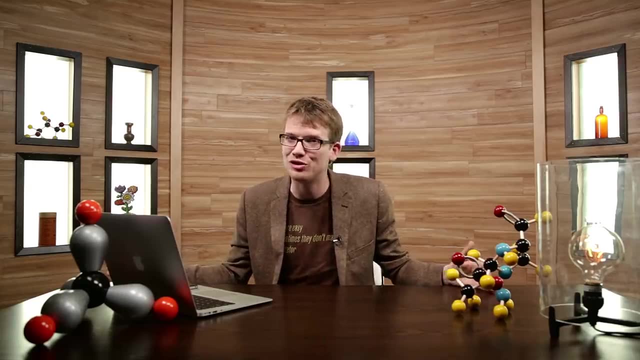 Unfortunately, it's next to impossible to know that number. It's too big and there are too many boxes where all that energy could be hiding. It's like trying to measure the total volume of the ocean. Like good luck, However, since energy 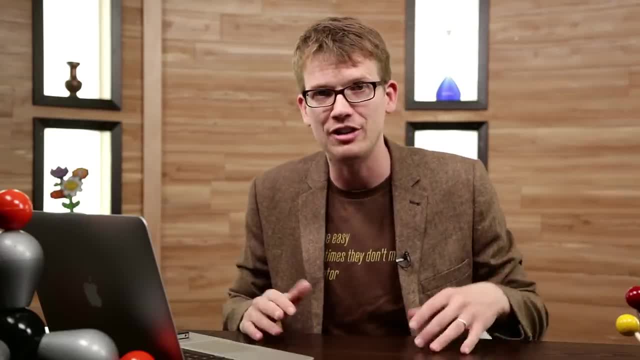 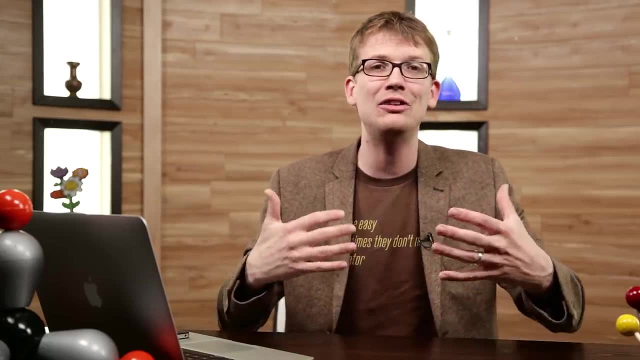 volume is a state function. we can very easily talk about the change in energy, Just like if you dump a two liter Mountain Dew into the ocean. you can't tell me how many liters are in the ocean, but you can say that that number has changed. 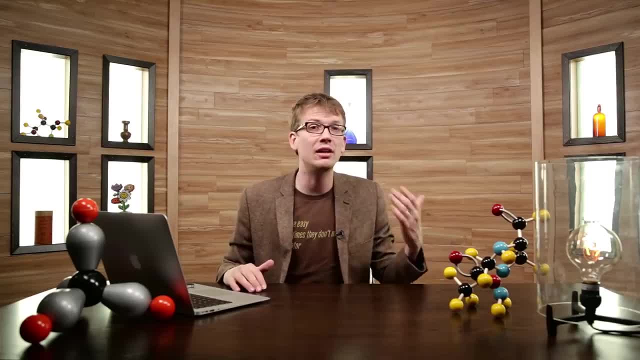 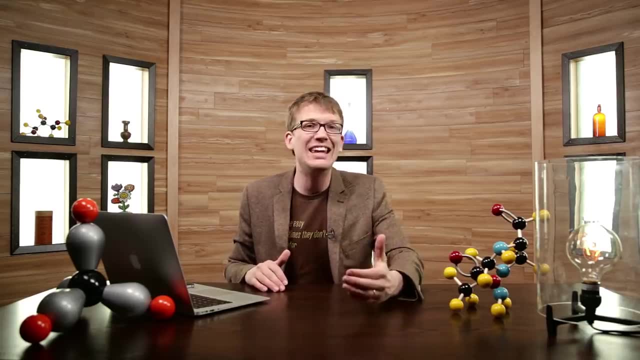 It has just increased by two. In the same way, we're interested in energy being transferred in or out of a system because of chemical reactions, And in many cases, all we're interested in is the heat part. For example, if I burn a pile of wood, I care about the heat being generated. 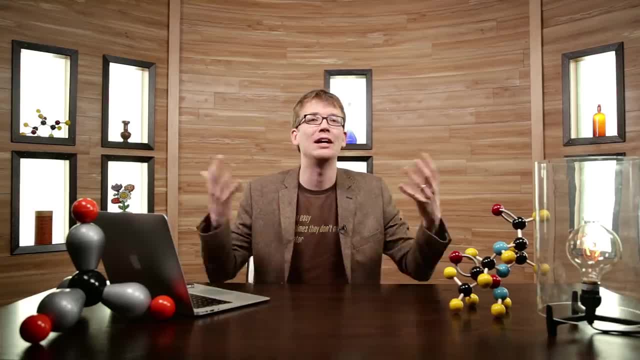 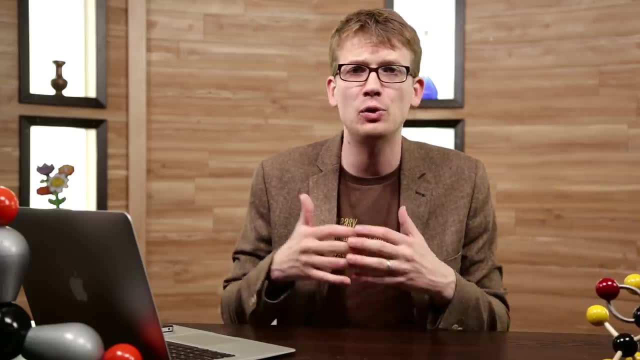 not the work being done by the volume increase or by the rising smoke. So dealing with the whole internal energy equation would kind of be overkill. What we really need is a state function based on the loss or gain of heat in chemical reactions, Which, yes, is what enthalpy is for. 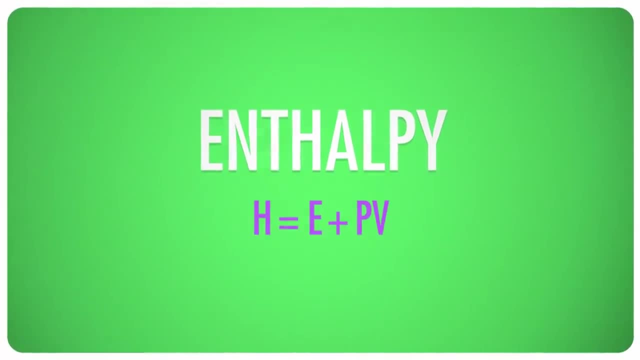 In addition to being a silly sounding word, enthalpy, which is represented by an equally silly capital, H, is technically the internal energy of a system, plus the energy that's required to sort of shove the surroundings out of the way and make room for the system's pressure and volume. 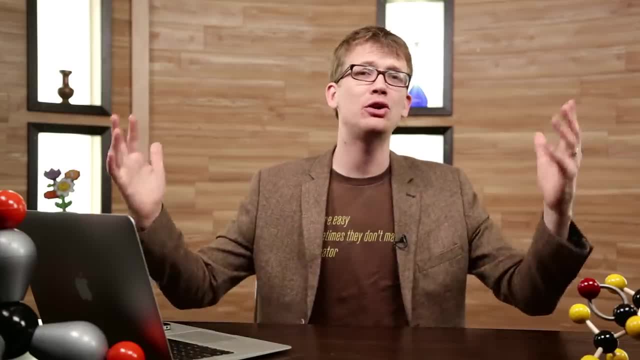 With enthalpy. we can make some assumptions and do some fancy math to make the simplest equation We've ever seen in Crash Course Chemistry. Let's get there real fast. So first, we're not really interested in the total enthalpy of the system. 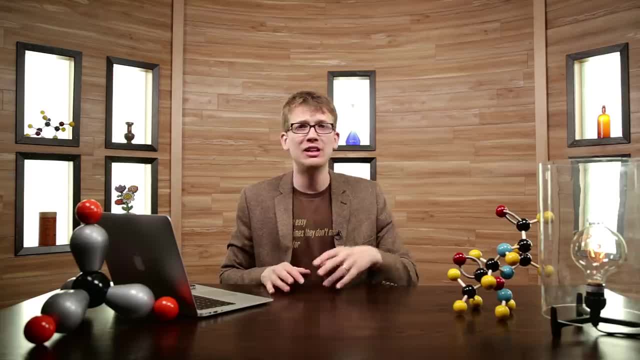 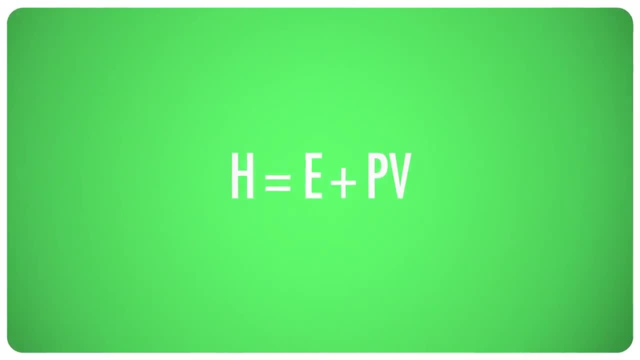 which is good, because it's impossible to measure. We're really just interested in how much it's going to change as a state function. So the formula for enthalpy is usually written as change in enthalpy. Delta E or change in energy equals Q plus W, so we can replace that part. 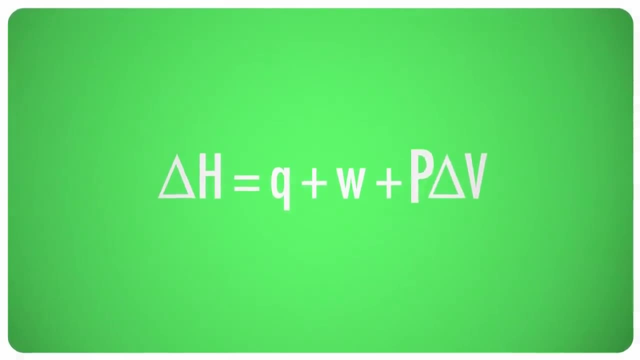 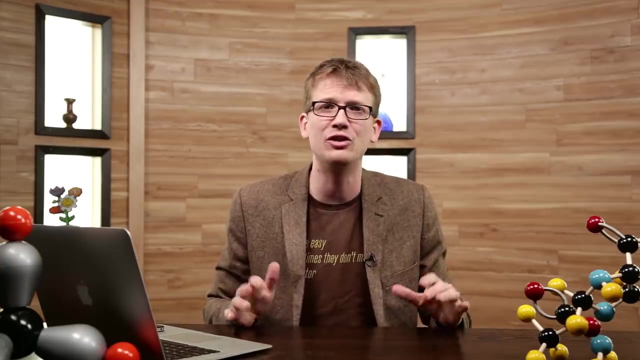 And then we can make two big, huge assumptions. First, that pressure is constant. Fortunately, despite talk of high and low pressure, weather systems, atmospheric pressure is really changes very little compared to the other terms in the equation. Constant pressure is a pretty good assumption here on the Earth's surface. 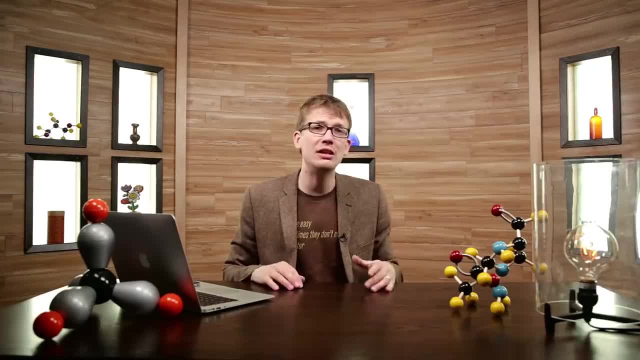 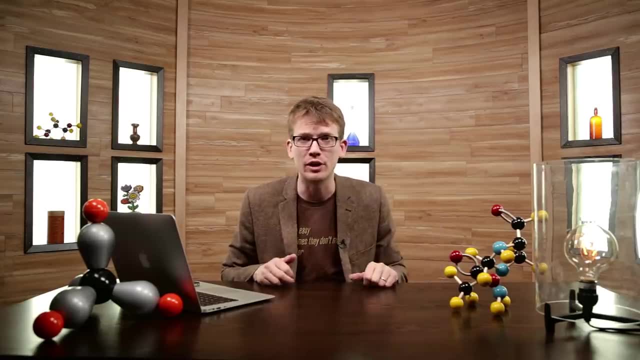 so that last delta only applies to the volume. The second assumption is that the only work done in the system is the work that the pressure does to change the volume, known as pressure-volume work. So W equals negative P, delta V. Now the signs are a little bit weird here. 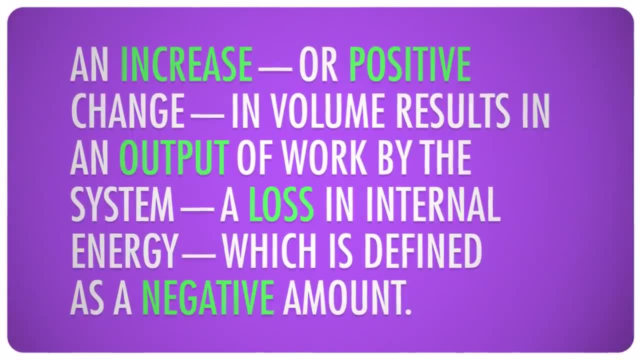 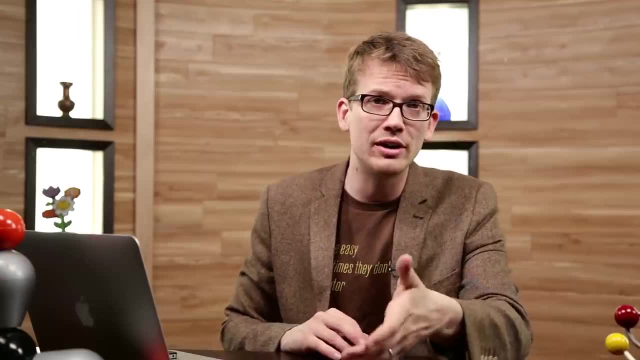 An increase or positive change in volume results in an output of work by the system, a loss in internal energy which is defined as a negative amount. So the signs for work and for P delta V will always be opposite, And so voila. 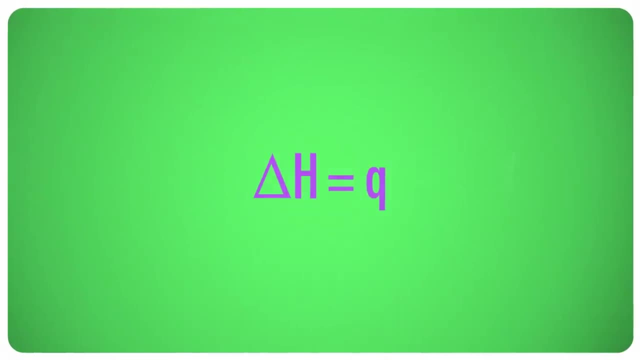 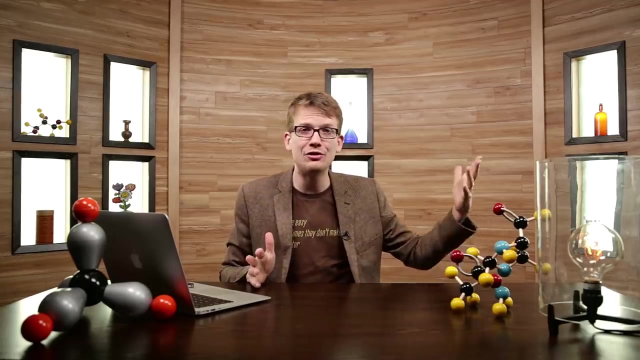 The P, delta V parts cancel. Delta H equals the heat of reaction. Change in enthalpy is equal to the heat gained or lost by the system. So I guess in the end the capital H for enthalpy does kind of make sense. 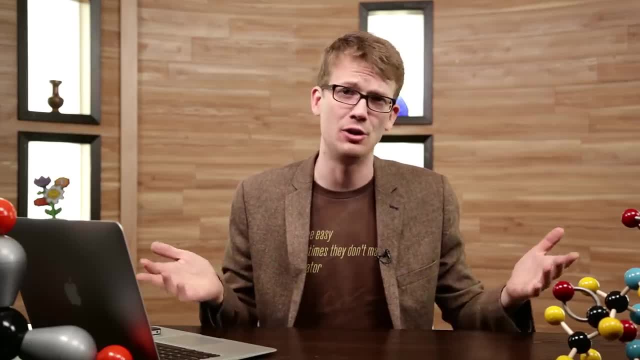 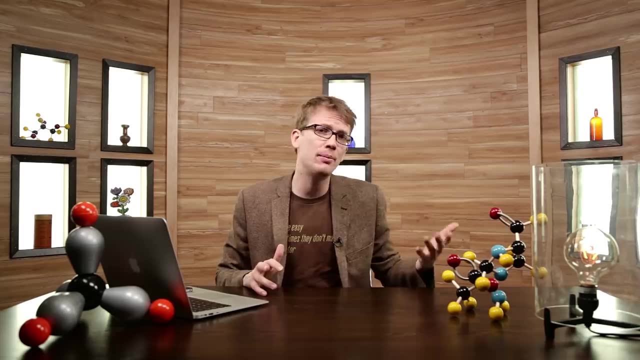 Thanks to this little trick, for a lot of reactions that happen at constant pressure, like here on the surface of the Earth, working just with enthalpies instead of internal energy makes a lot more sense. I mean it's hugely useful. We can determine how much. 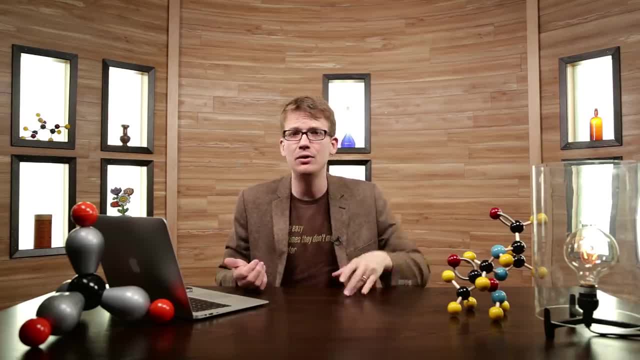 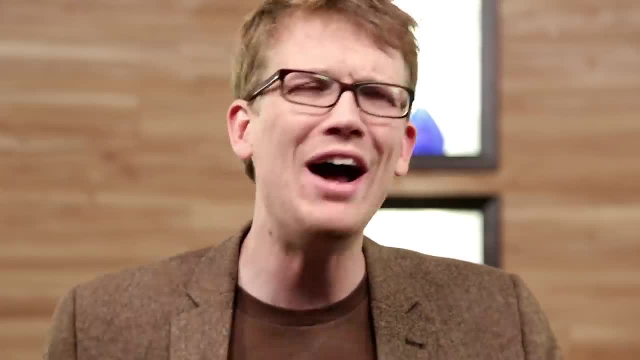 useful energy is contained in pretty much any chemical compound. This is done by simply measuring temperature changes during chemical reactions. So we know what it is. We know that state functions are great, But really why? Why have we done this? And can I just go look at pictures of cats now? 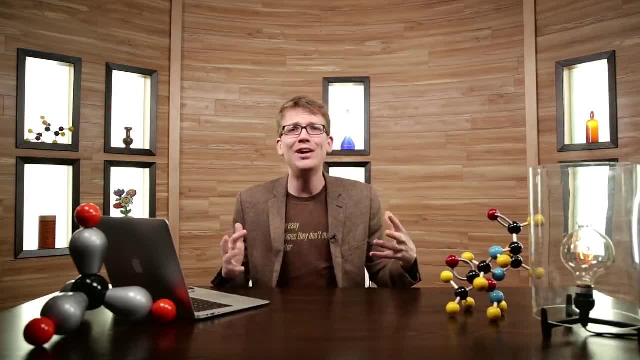 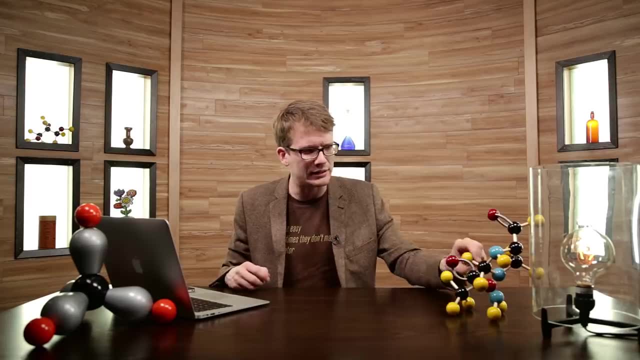 Well, no, Because you don't even know why enthalpy is so cool. When a reaction takes place and enthalpy changes, that heat is transferring into or out of actual chemical bonds, These little guys, Atoms and molecules, reacting so that they contain more or less energy. 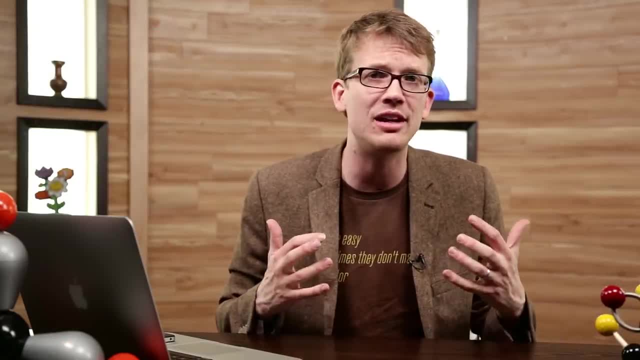 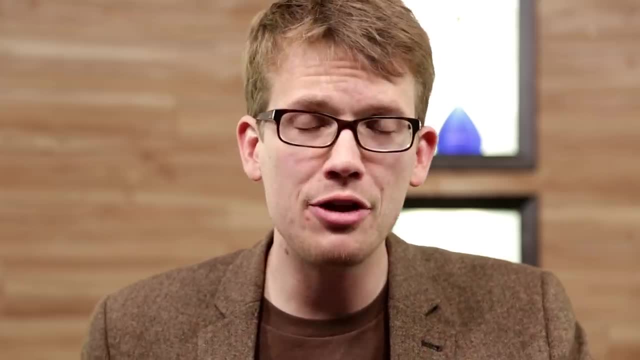 And that energy is either released to or taken from the environment as heat. Those bonds are nothing but energy, And using enthalpy we can measure how much energy they have. And we measure enthalpy with a weird little science called calorimetry. 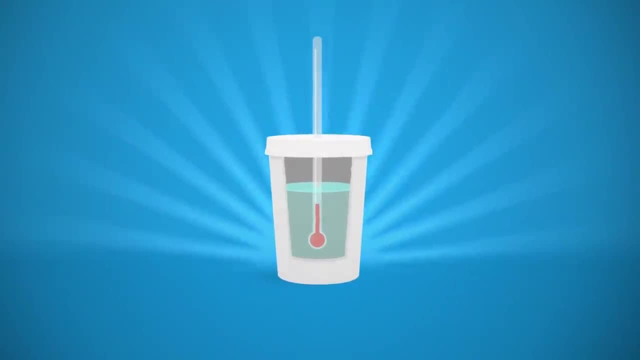 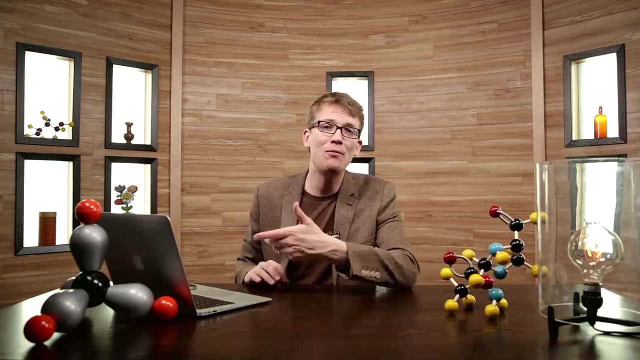 In calorimetry we have a reaction take place inside an insulated vessel, like the thermos basically, and measure how much the temperature changes, which we can then link directly to heat and thus enthalpy change. Hopefully that sounds like fun. 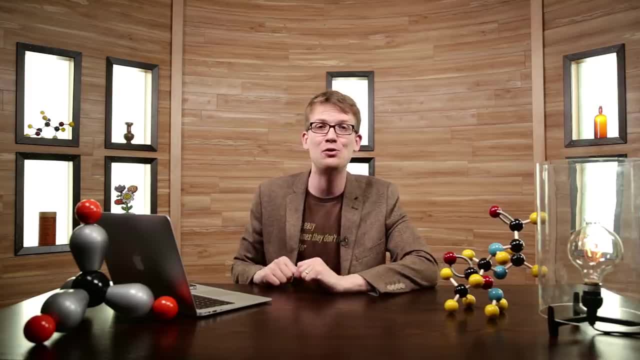 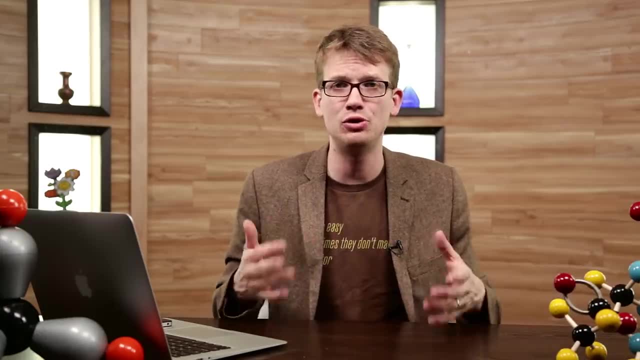 because more about the ins and outs of this are coming in an episode on how to measure enthalpy. Scientists have actually done a lot of the calorimetry footwork for us, so we can actually predict how much heat a chemical reaction will produce. 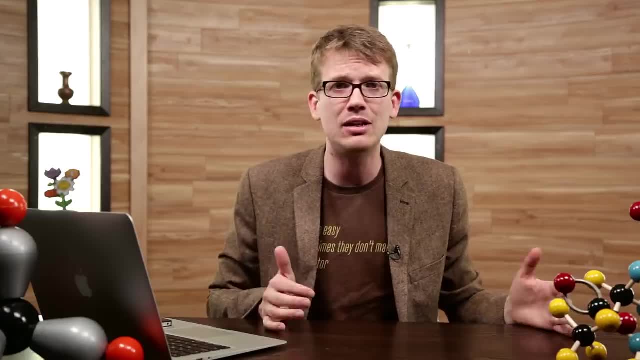 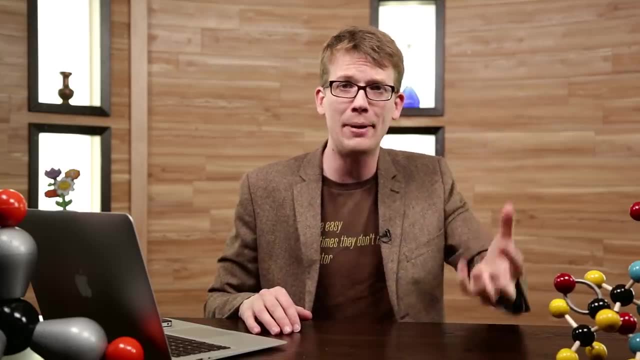 You might not understand what's so great about that, but just imagine, because I live here in Montana, where winters are pretty wintery, I can invent a hand warmer just by doing some calculations on paper, without driving to Texas to buy the stuff and do all kinds of expensive experimenting. 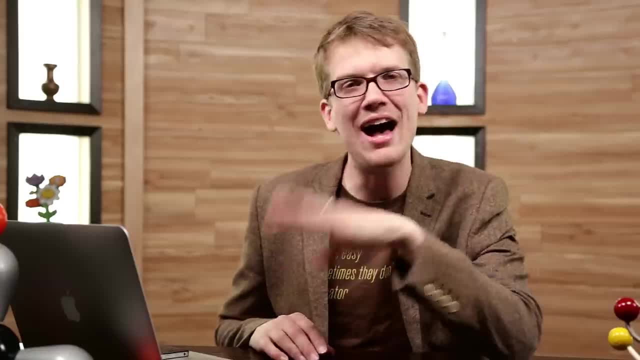 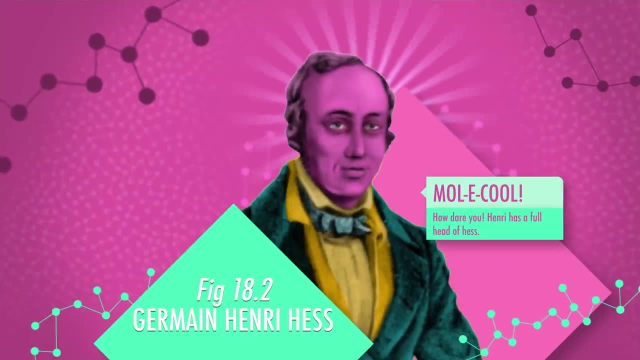 For that we have to thank good old Sherman Hess. No, not Herman Hess the gaunt balding Swiss author and poet, but Sherman Hess, the gaunt balding Swiss author and chemist. Yeah, even the history parts of chemistry are confusing. 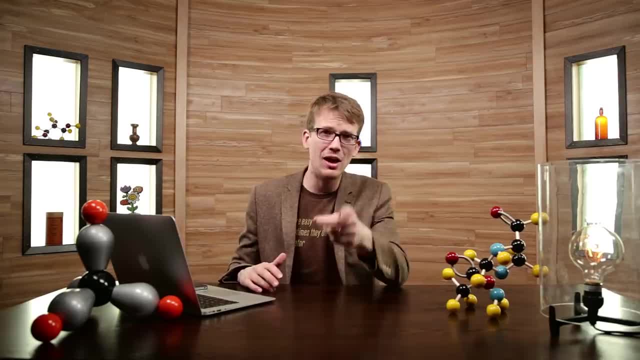 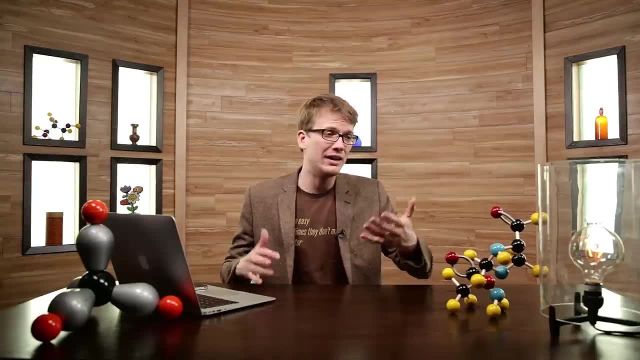 Hess was a chemist, geologist, professor, author, a doctor, and he also got a law named after him, which is pretty much the highest honor you can get as a chemist. Hess's Law, which also kind of led directly to the first law of thermodynamics. 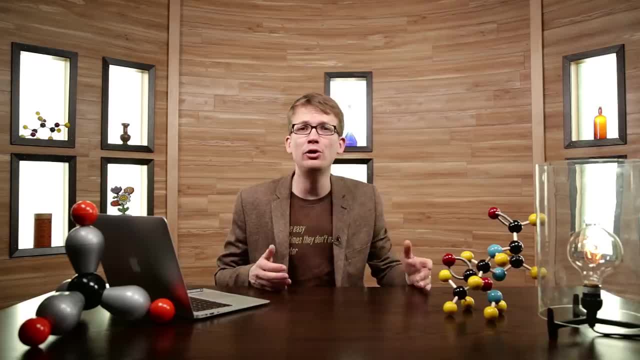 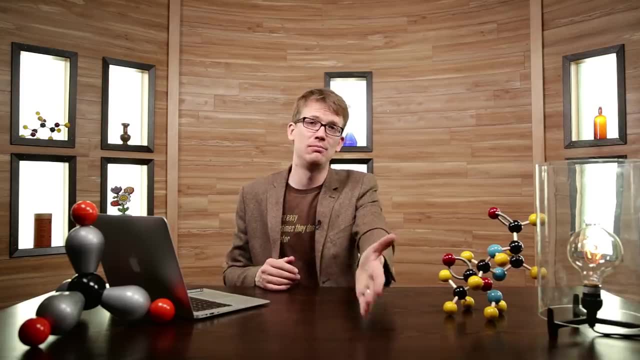 Kind of a big deal, Not bad. Hess's Law says that the total enthalpy change for a reaction doesn't depend on the pathway it takes, but only on its initial and final states. Sounds pretty familiar, right, As long as you start with the same reactants and end with the same products. 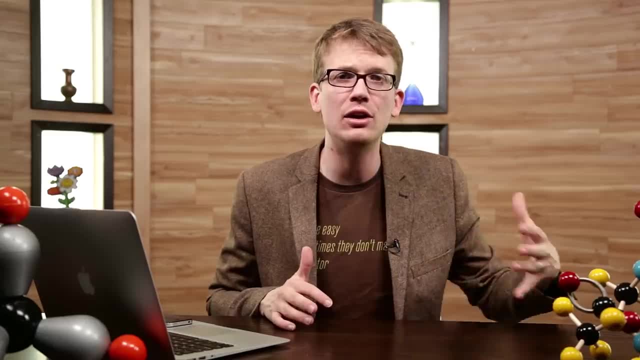 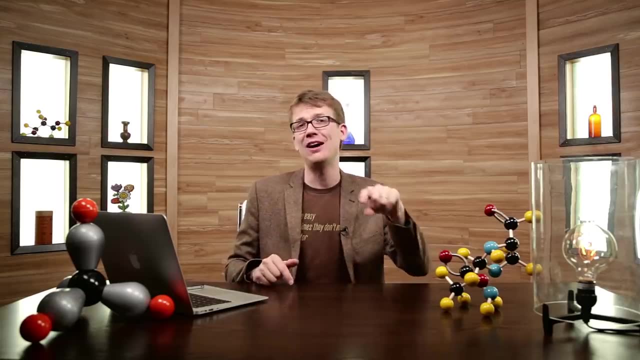 the enthalpy change is the same. In order to study this stuff carefully, he looked at the standard enthalpies of formation of the reactants and the products of a reaction. To define standard enthalpy of formation, I'm first going to define what a standard state is. 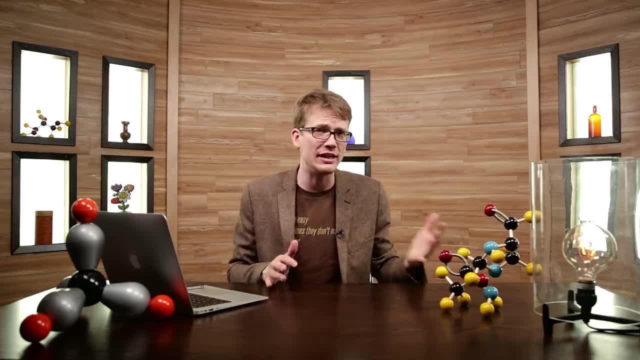 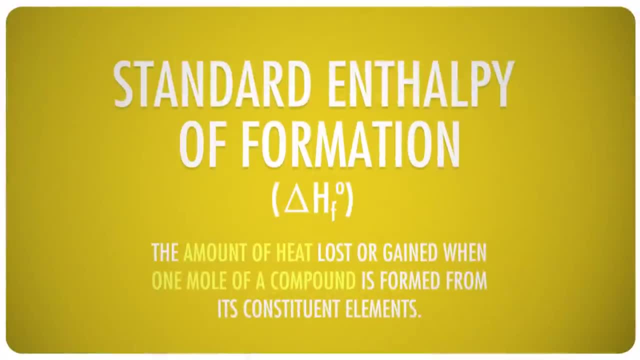 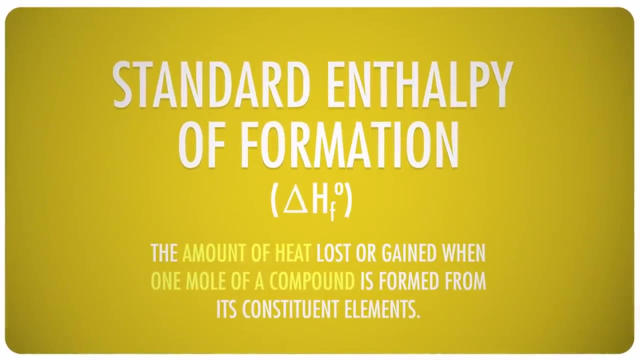 Basically it's just a set of criteria so that chemists can all be studying stuff under the same conditions. Chemicals in their standard state are at 25 degrees Celsius and 1 atmosphere. Standard enthalpy of formation is the amount of heat lost or gained when one mole of a compound is formed from its constituent elements. 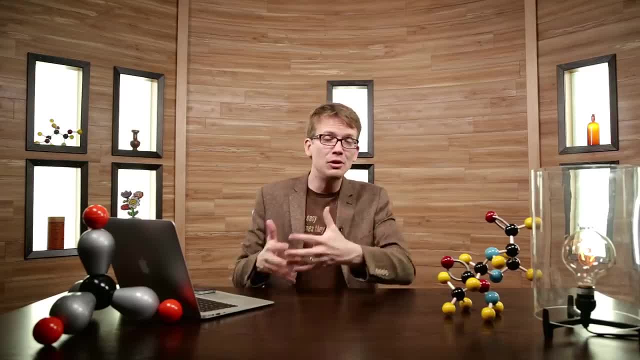 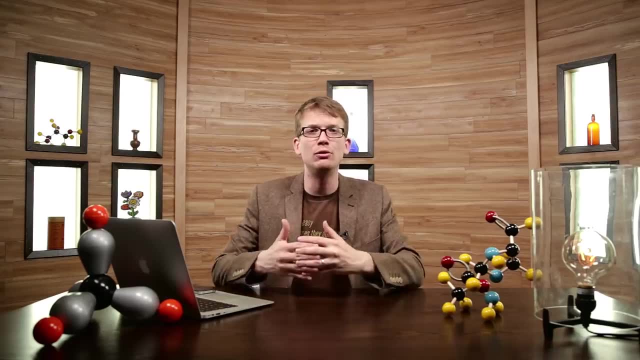 And, of course, all of those elements have to be at their standard states. Since absolute enthalpy is unknowable, though, we have to be measuring from a baseline, And that baseline is the individual element's most stable form. at standard state, That most stable form is defined as zero. 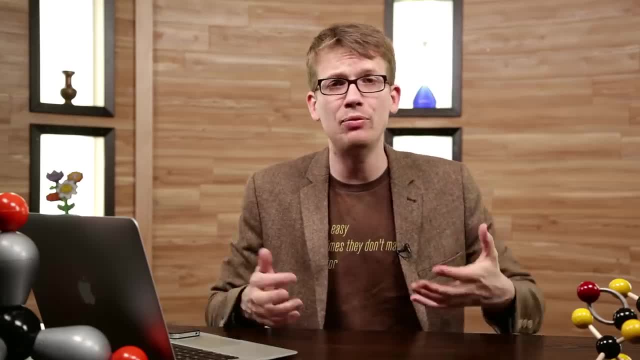 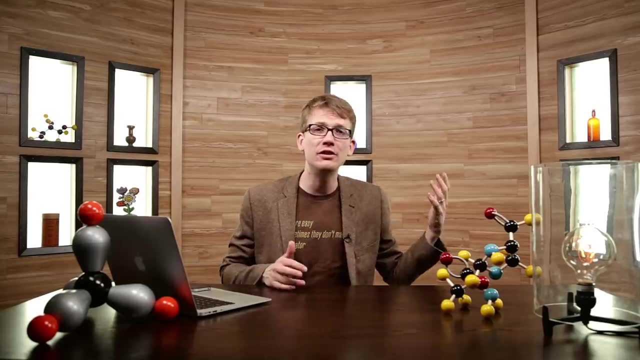 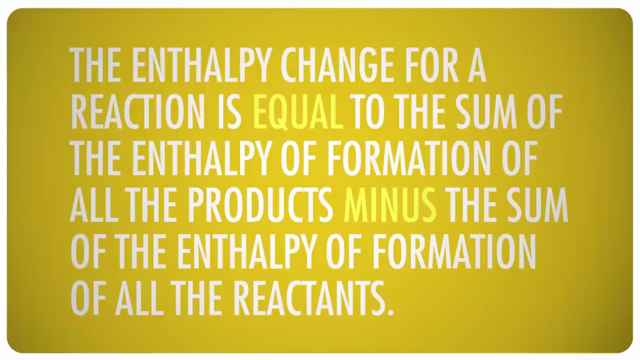 Values for compounds are measured from that zero baseline, and then the standard state values can be used to calculate the enthalpy change for any reaction, even hypothetical ones. Hess's law is often stated in terms of standard enthalpies of formation. The enthalpy change for a reaction is equal to the sum of the standard enthalpies of formation. 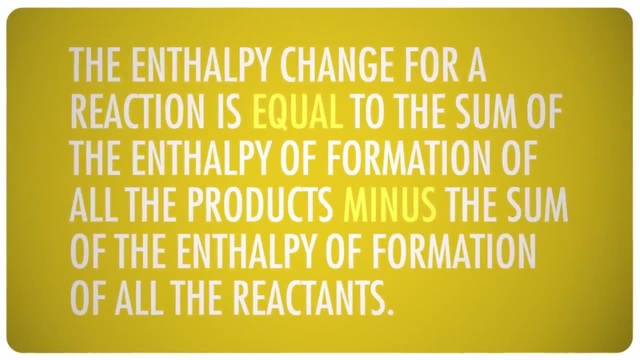 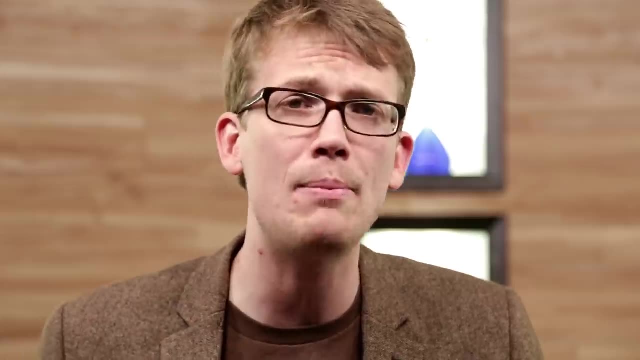 of the products minus the sum of the standard enthalpies of formation of the reactants. Thanks to many hardworking chemists, the standard enthalpy of formation has been measured for hundreds of compounds. We can just look them up in charts and plug them into Hess's law. 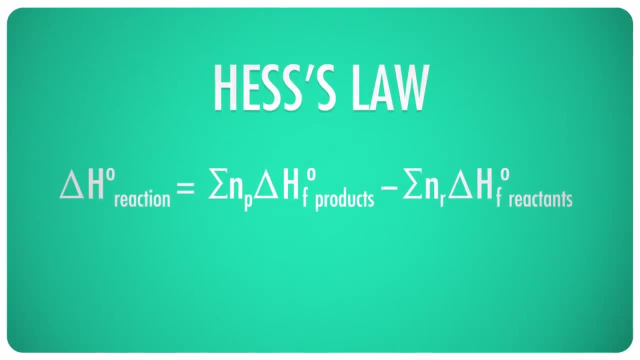 Speaking of which, here is Hess's law as a mathematical formula. Pretty fancy looking, but it says exactly the same thing. The enthalpy change for a reaction equals the sum of the standard enthalpies of formation of the products minus the sum of the standard enthalpies of formation of the reactants. 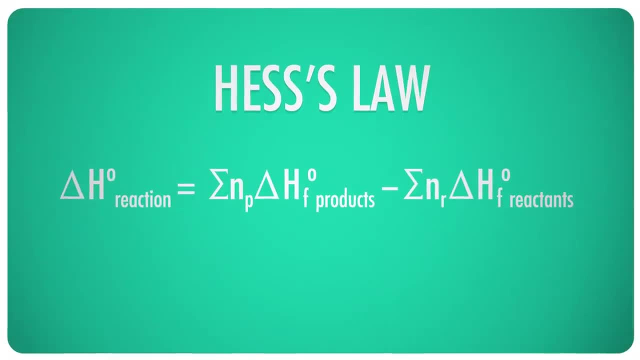 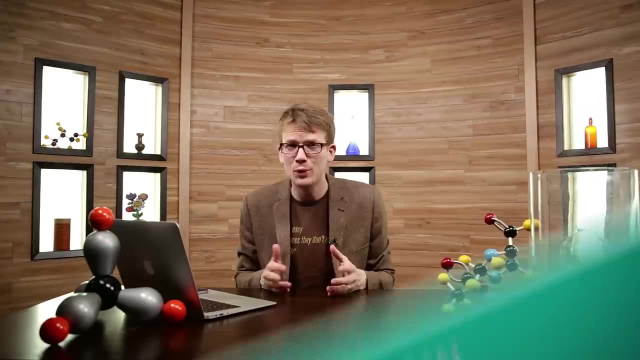 That pointy little funny E-looking thing is the capital Greek letter sigma, and it means the sum of Np and nr are the moles of each product and reactant respectively. We have to factor that in because, remember, the standard enthalpy of formation is measured for just one mole of the substance. 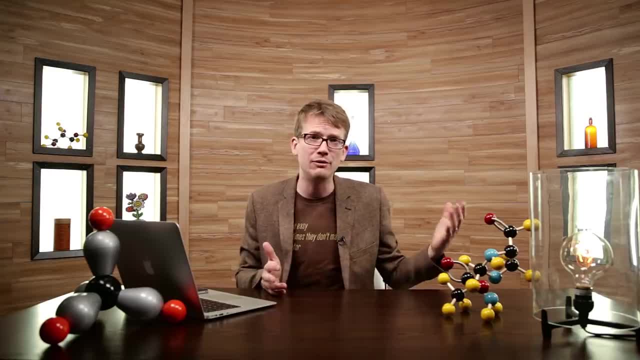 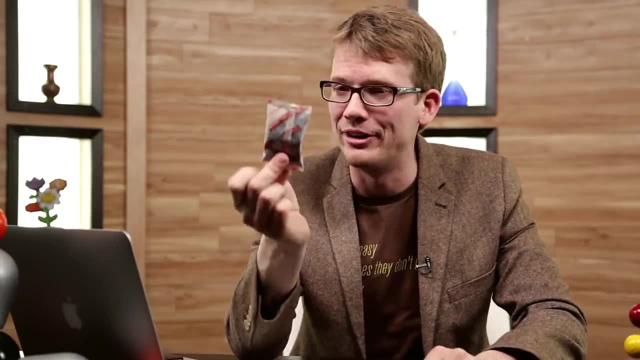 If the chemical equation uses more than that, we have to multiply the standard enthalpy of formation by the number of moles in the equation. Again, I have just the thing for the calculating Exhibit A, a hand warmer. It gets warm because of an exothermic chemical reaction. 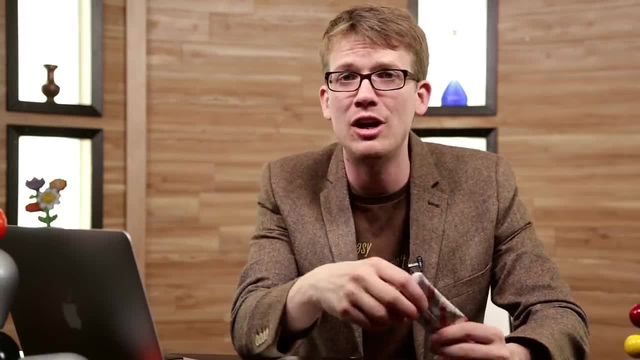 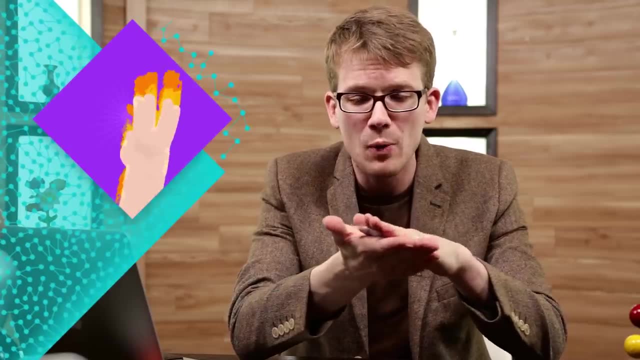 and I'm very happy. the inventors knew how to calculate the enthalpy change of chemical reactions. They chose one that releases just enough heat quite slowly to heat up my hands nice and warm without burning them off. The reaction combines an iron powder. 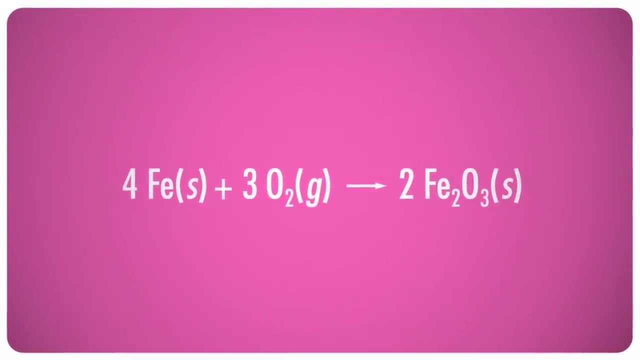 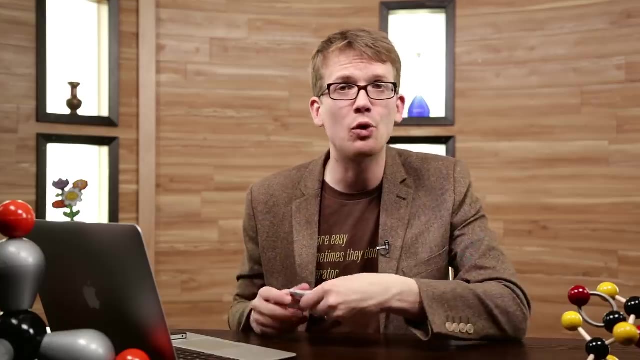 which is in here, and oxygen which diffuses through the membrane of the little packaging. It forms iron oxide, the main ingredient in rust. To calculate the enthalpy enthalpy change of the reaction or heat of reaction, we simply find the delta HF of all of the reactants and products. 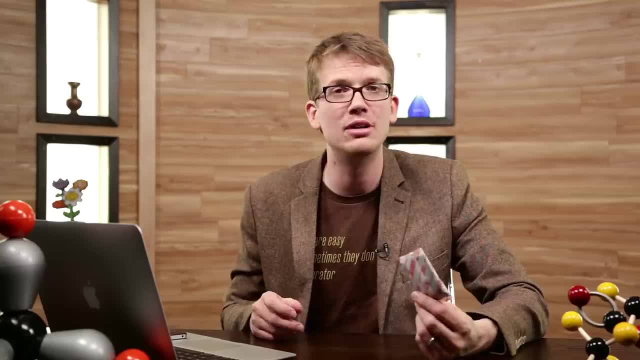 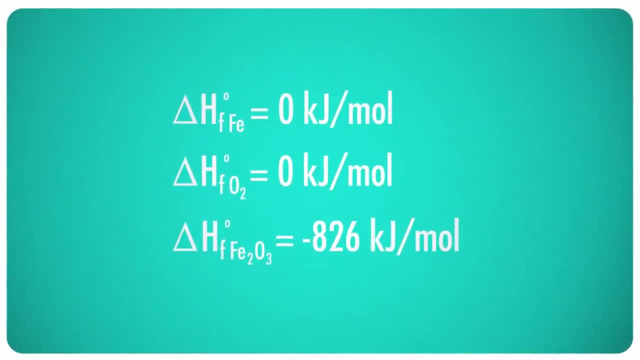 either in the back of most textbooks or on Google and plug them into Hess's Law. Delta H of formation of elemental iron and oxygen are zero by convention. When in doubt, find them in the same table, And the delta H of formation of iron oxide is listed as negative: 826 kilojoules per mole. 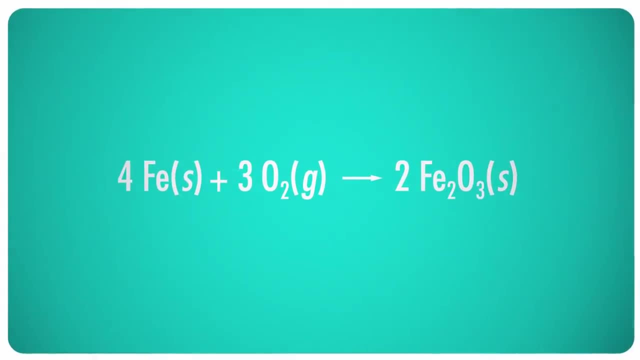 First, we have to make sure that we have balanced the chemical equation. so do that number one. Second, let's look at Hess's Law and figure out what our products are and what our reactants are, and stick them in. 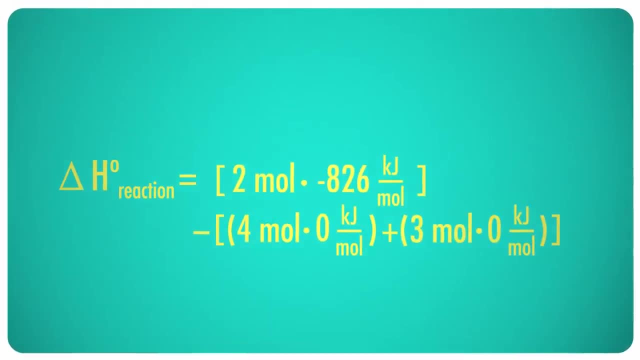 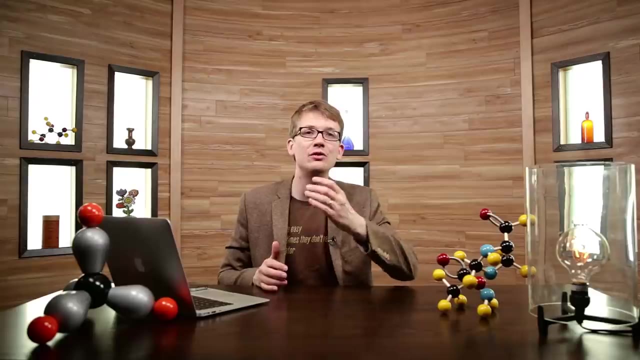 Then plug in the number of moles for each of our products and reactants, Bang on your calculator and realize the delta H of the reaction is negative, 1652 kilojoules. So the reaction of four moles of iron powder. 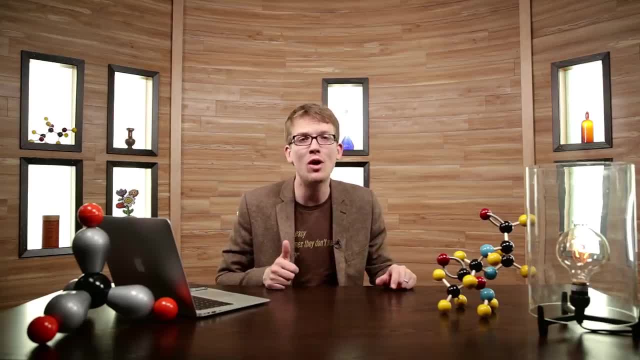 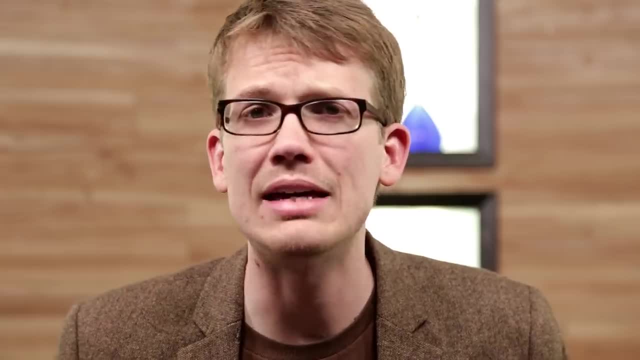 which is about 223 grams of iron, releases 1652 kilojoules of heat. All that energy locked away in chemical bonds and then released as heat to my aching, frozen fingers. Better living through chemistry. Thank you for watching this episode of Crash Course Chemistry. 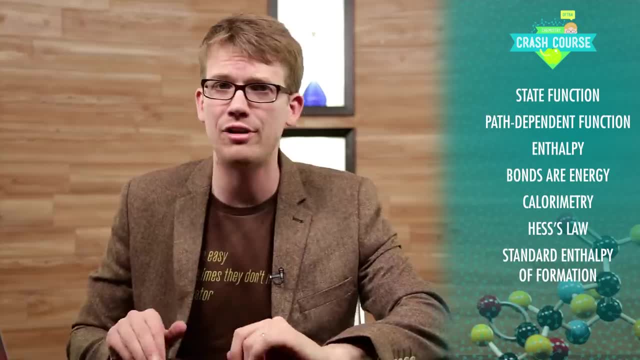 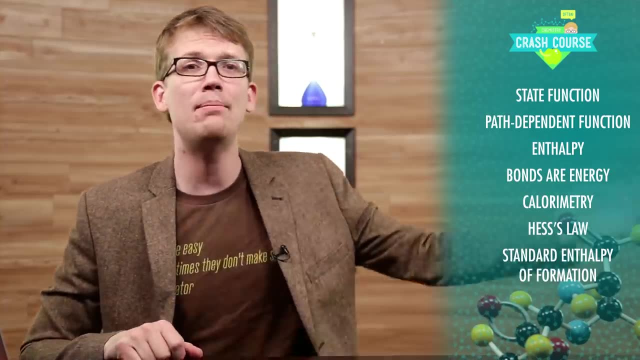 If you were paying attention today, you learned what the state function is and how it varies from a path-dependent function, why enthalpy change is different from heat, even though they turn out to be pretty much the same anyway- that bonds are energy.